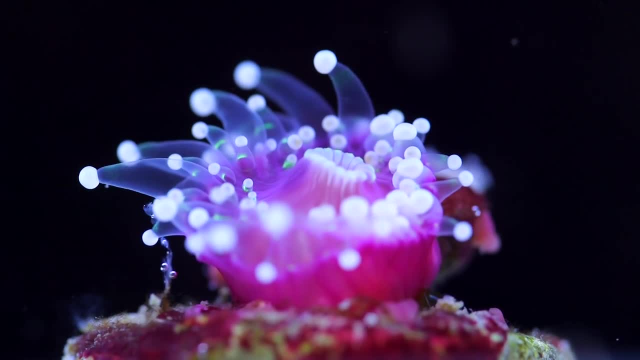 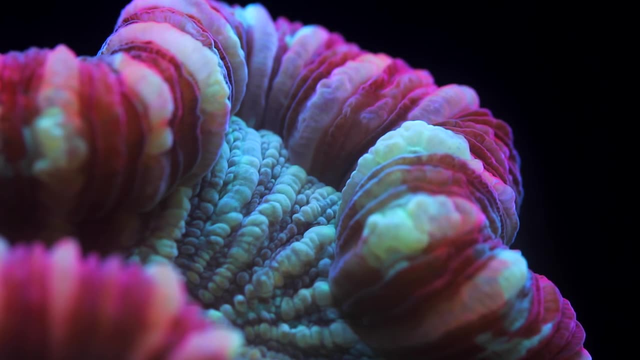 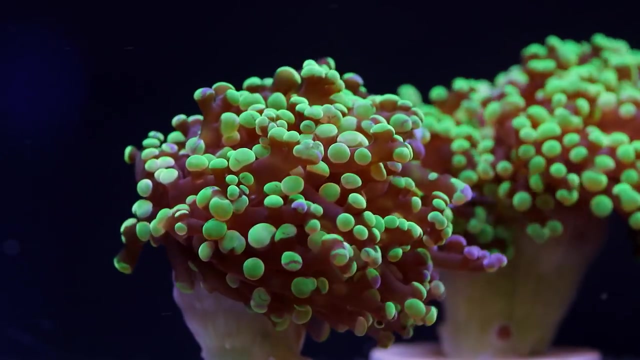 and the thing that's going to most dramatically affect how fish and coral look in your tank. My goal in making this video isn't so much to give a primer to beginners. it's more to illustrate just what a difference lighting can make. Corals can color up differently. 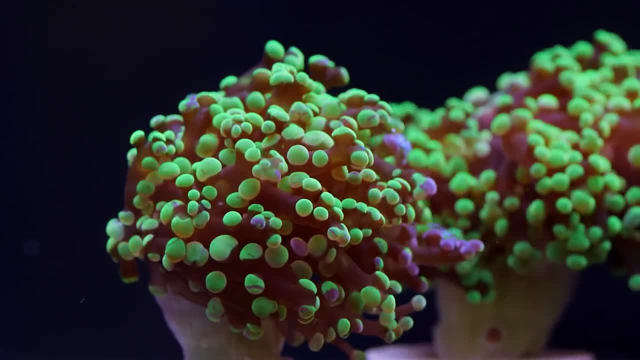 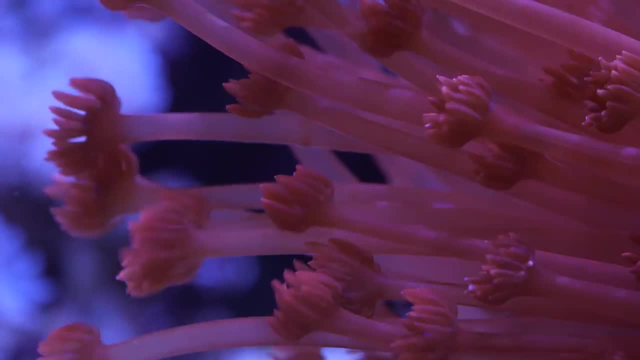 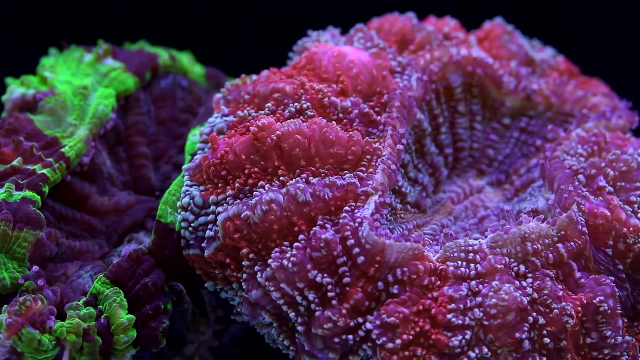 under different lighting systems to varying degrees, but lighting systems can also drastically affect the appearance of the same exact coral. A lot is made of what corals look like online. Are the images over saturated? What kind of lighting was taken under? What will it look? 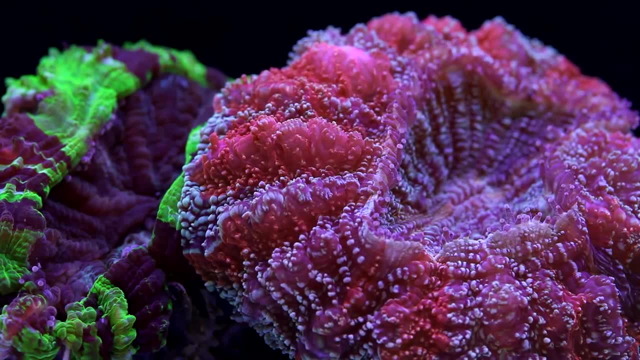 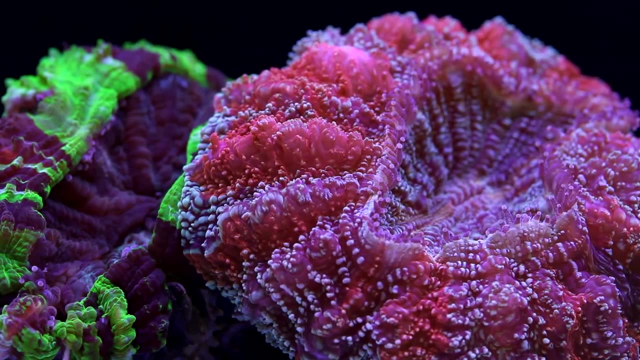 like in my tank. The list of questions goes on and on. What most people don't really realize is that much of what that coral will look like has more to do with the lighting selection by the hobbyist than the image of the coral online. 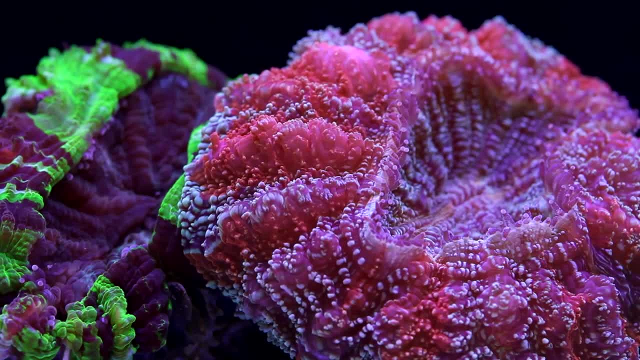 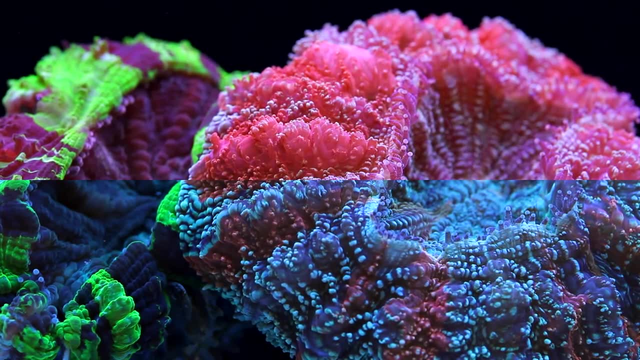 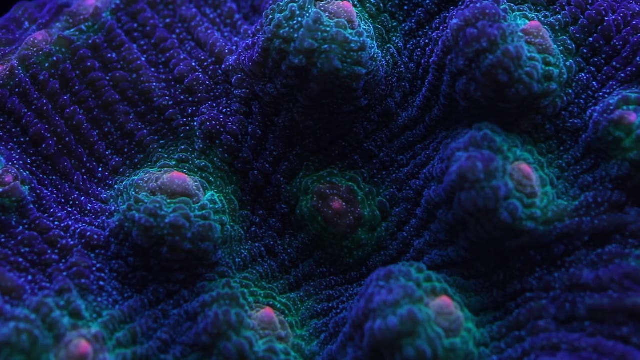 Obviously, there's pictures online that look way off, but, assuming for a moment that the picture is good, there is a really good chance that any coral is going to look very different from tank to tank depending on that light. I tried to show the corals on my site and during live shows under different types. 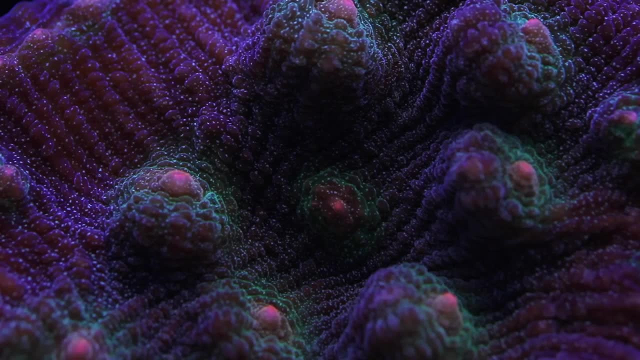 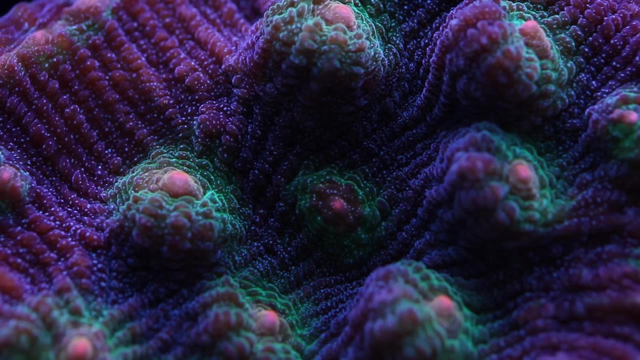 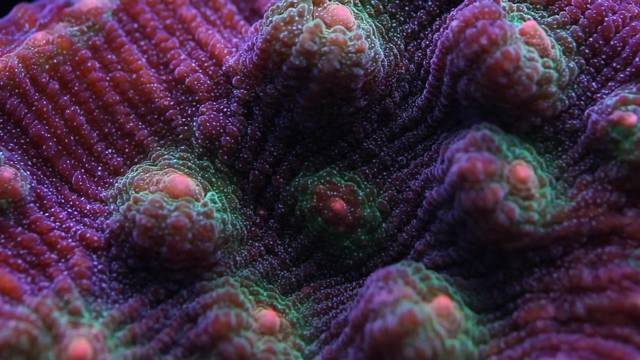 of lighting, but these things are just helpful guidelines at best. In the background, you're going to see some corals illuminated under different types of T5 bulbs. Moving from T5 to a different technology altogether, such as LED or metal halide, will have an even more pronounced difference. 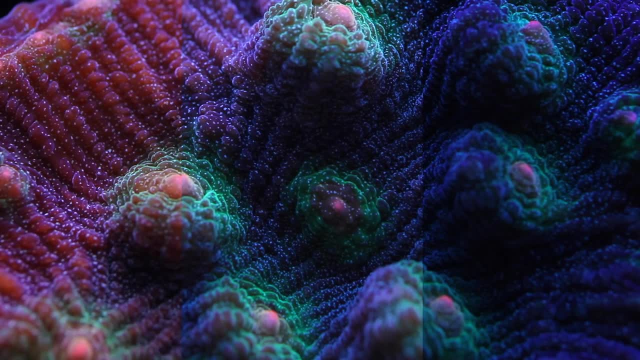 In the background you can see some corals illuminated under different types of T5 bulbs. moving from T5 to a different technology altogether, such as LED or metal halide, will have an even more pronounced difference. In the clip I just showed, I transitioned from a full actinic look to an almost full 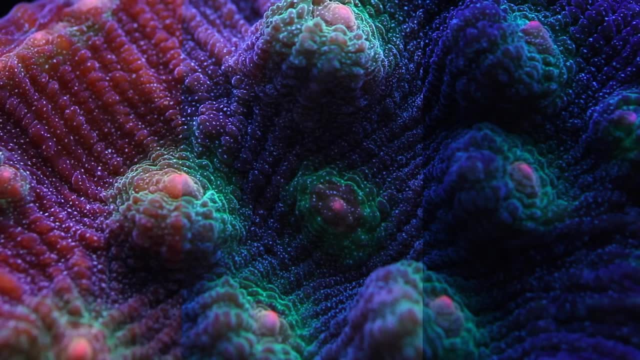 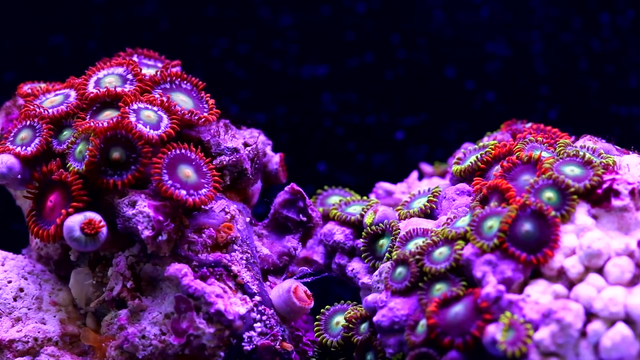 daylight. look by changing lights. Go back and take a look. if you didn't notice the first time around Here you can see three slices of the same coral under those different lights. One might think that the solution to this is to only shop in person for corals. 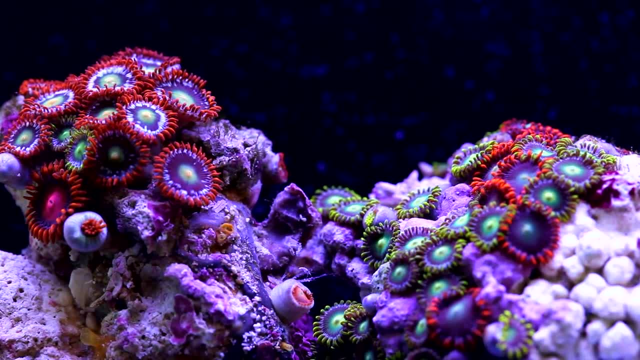 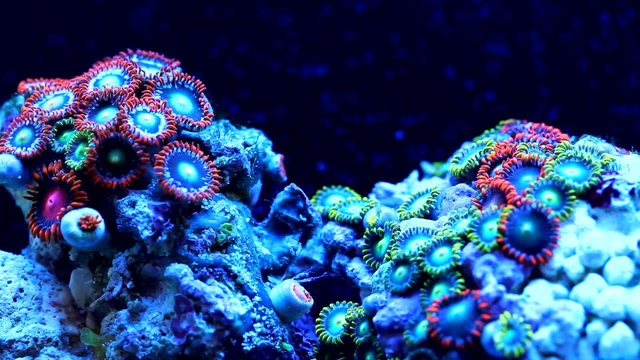 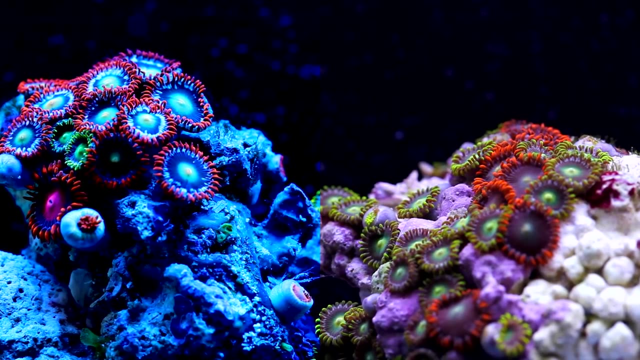 I try to do that as much as possible. however, nothing is 100%. I have purchased corals in person that looked spectacular. One in particular looked really special. It was glowing red and yellow. The yellow drew my eyes right to it and I decided to purchase it.